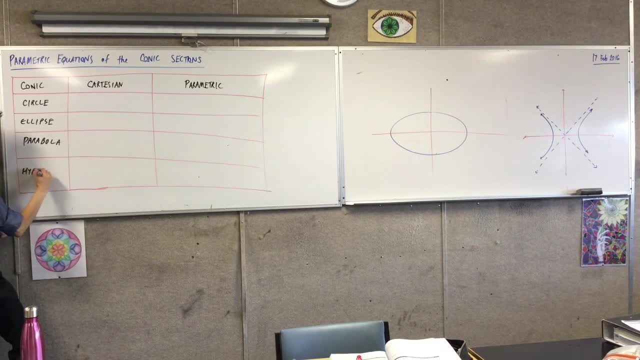 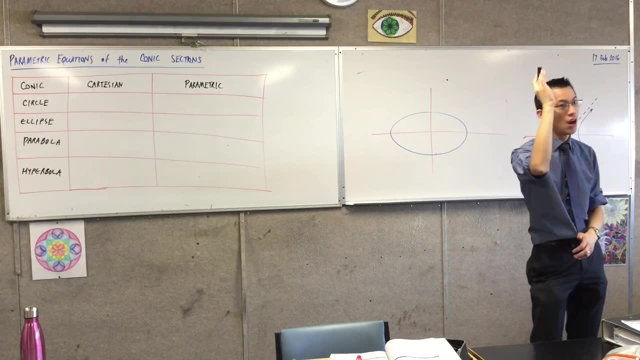 And then the hyperbola is what happens when, on the cone, which is actually a double cone- when you go sufficiently far enough that you don't just get one branch, one intersection, one section of the cone, you actually wind up hitting the other side, and that's why there are these two branches. 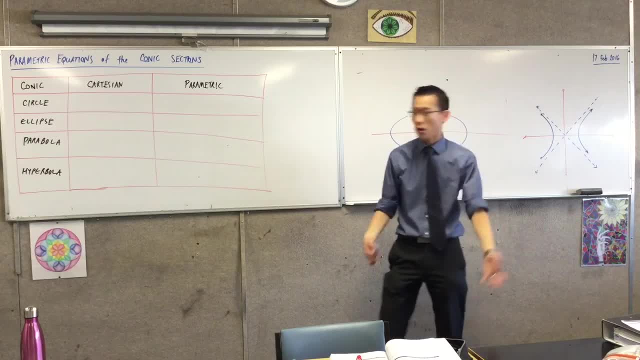 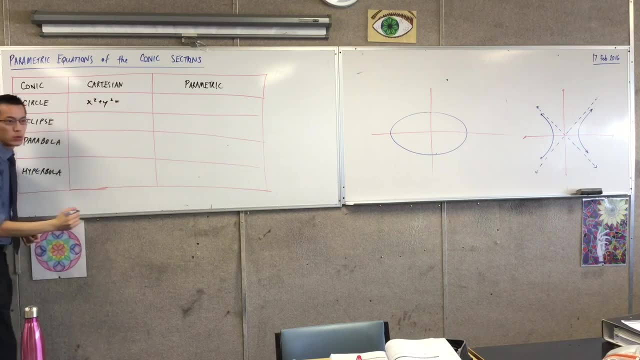 So let's think about the Cartesian equations for all these, because we know all of these And we'll just do some standard forms. So let's do this. So, for instance, here we have: x squared plus y squared equals 5.. 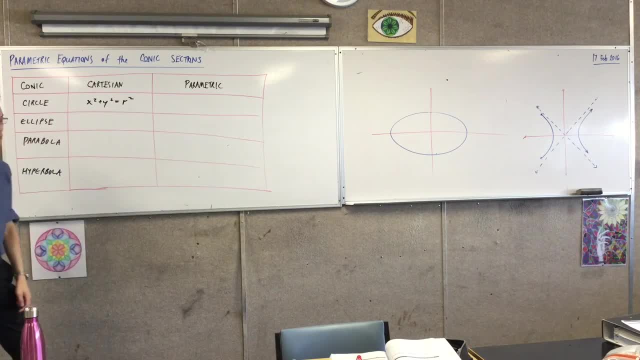 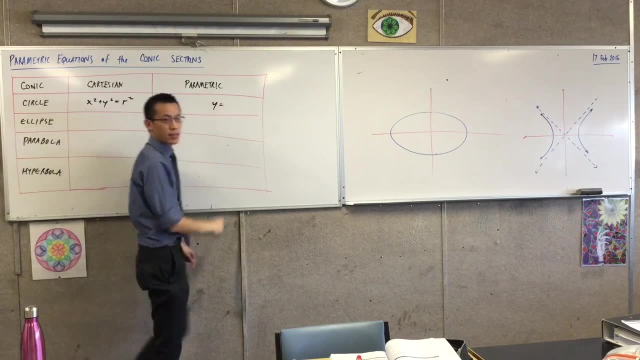 Now we would usually say r squared right, r squared because it's the radius. Now we know the parametric equations for this circle. Parametric equations are equations for x and y that connect us back to that single variable, whatever that may be. 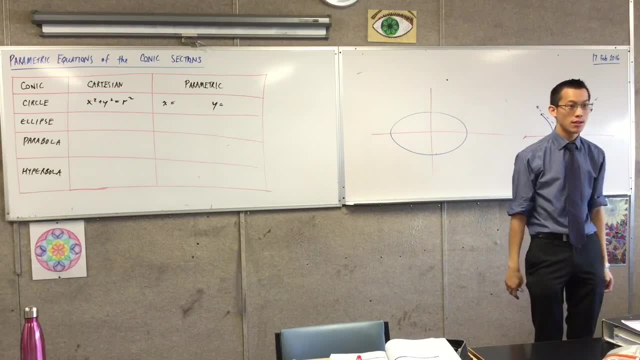 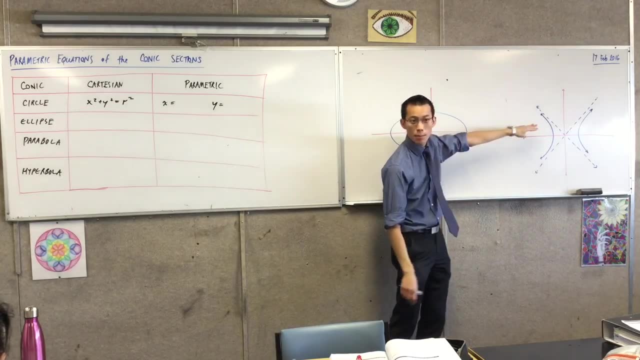 Now, what variable do we choose as a parameter for the circle? We chose an angle measured at the centre, at the origin, From the point against the positive x-axis. It's very important we define what that is. So then we said, okay, well, if I've got a radius of r, this is not the unit circle, right? 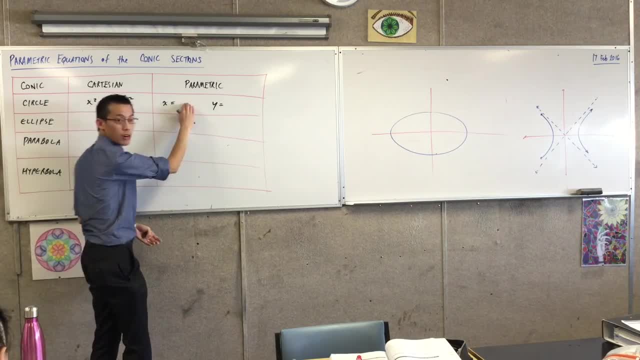 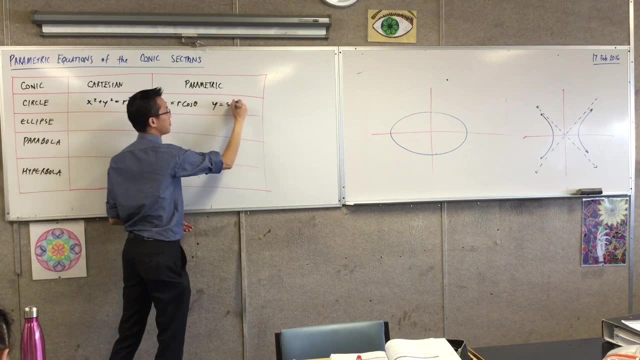 I mean, it might be, but we don't know. So therefore, instead of just cos theta sine theta, I have to account for the fact that I'm r times further away from the origin, So that's where we get this from. 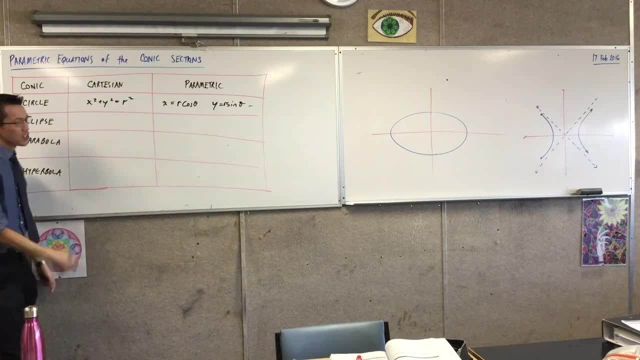 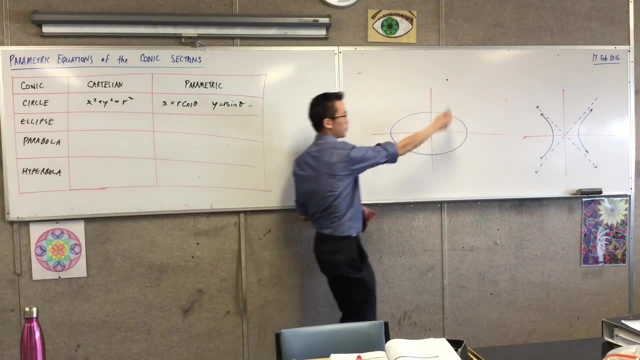 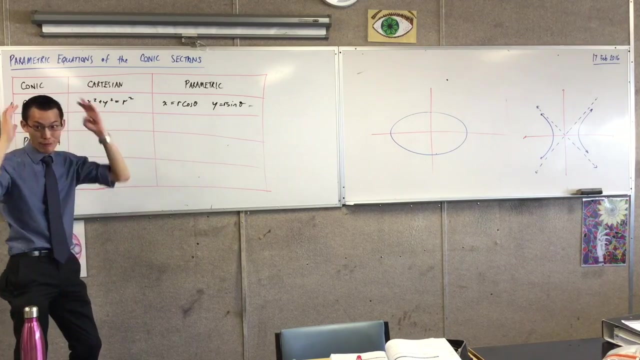 Like. so, Also important to mention, there's kind of a range restriction on theta right. It can't just go anywhere, Because once you go like around a full revolution, you've come back to where you started, right. So therefore, I guess the way I would say this is as an extension to students thinking in gradients rather than in degrees. I can go from 0 to 2 pi. That's one full revolution. I mean, in theory, there's nothing stopping you from going past 2 pi, But the whole point is to have one unique defining factor for where you are on your locus, right. 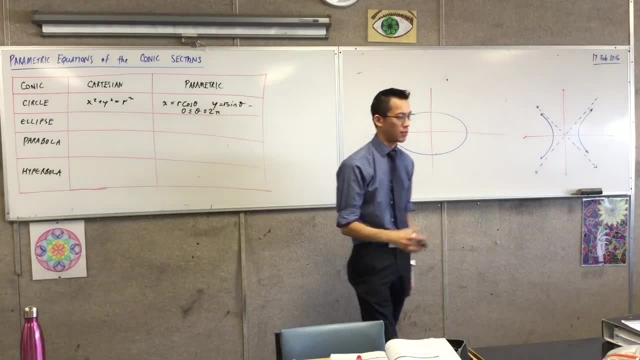 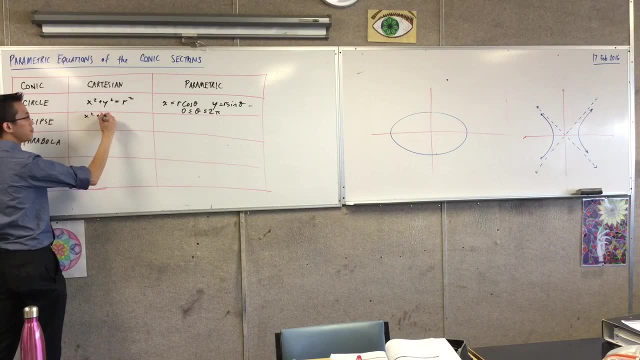 So, therefore, if I restrict it from 0 to 2 pi, everything is unique, Uniquity, Uniquity. Okay, So when we go to the ellipse, what changes? Okay, We still have the x2 plus y2.. 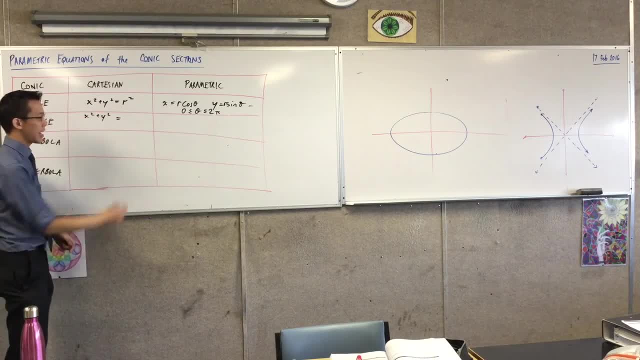 But we don't frame it in these terms, do we? We tend to say: well, there's a 1 over here, And then we get some denominators And we have different denominators, generally speaking, Because if you don't have different denominators, you'll back up in circle territory. 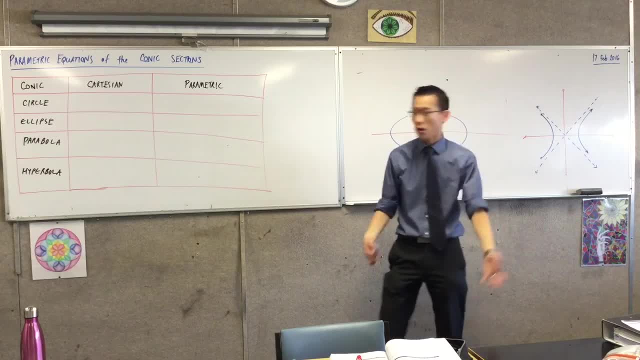 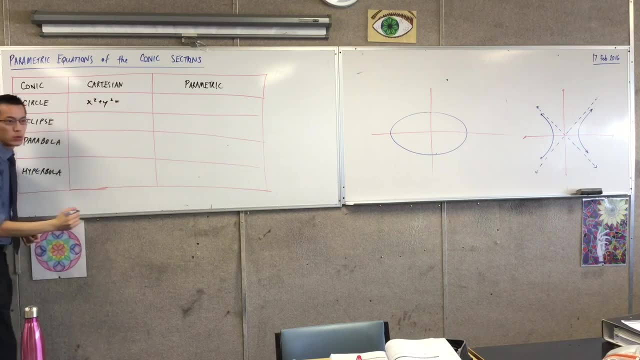 So let's think about the Cartesian equations for all these, because we know all of these And we'll just do some standard forms. So let's do this. So, for instance, here we have: x squared plus y squared equals 5.. 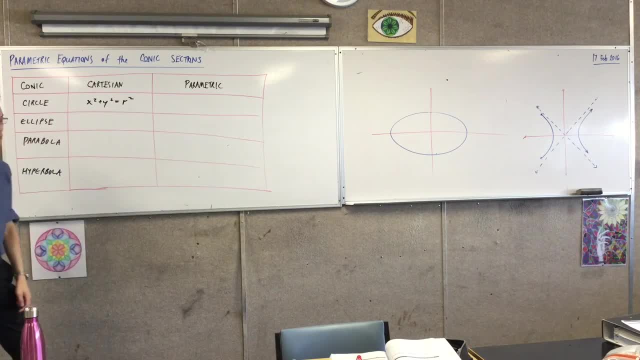 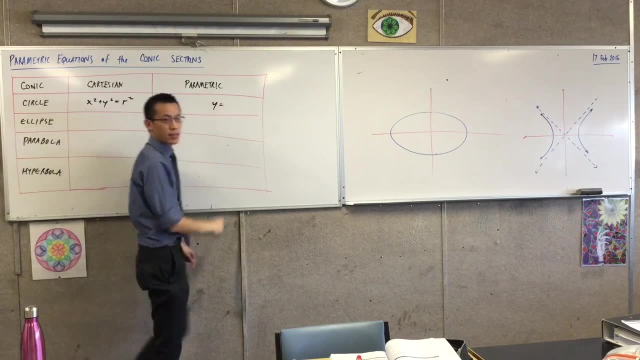 Now we would usually say r squared right, r squared because it's the radius. Now we know the parametric equations for this circle. Parametric equations are equations for x and y that connect us back to that single variable, whatever that may be. 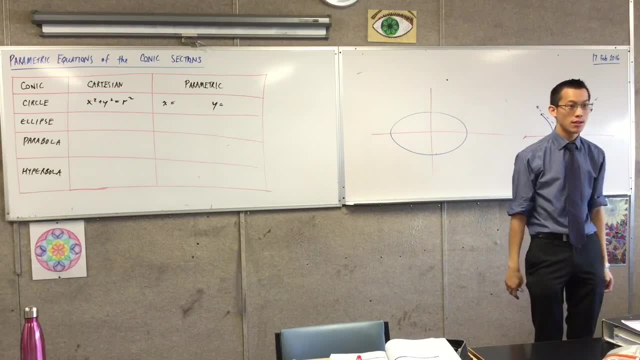 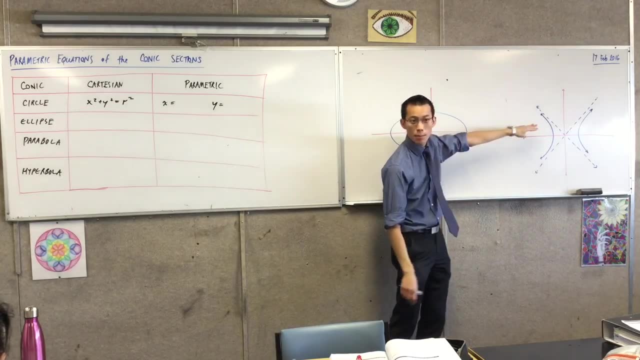 Now, what variable do we choose as a parameter for the circle? We chose an angle measured at the centre, at the origin, From the point against the positive x-axis. It's very important we define what that is. So then we said, okay, well, if I've got a radius of r, this is not the unit circle, right? 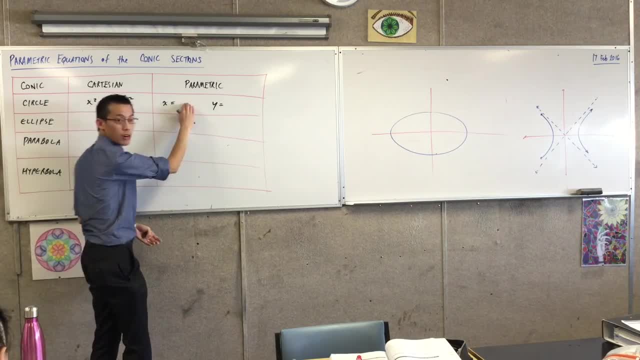 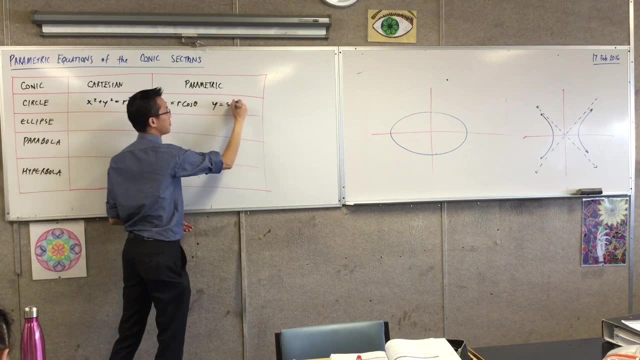 I mean, it might be, but we don't know. So therefore, instead of just cos theta sine theta, I have to account for the fact that I'm r times further away from the origin, So that's where we get this from. 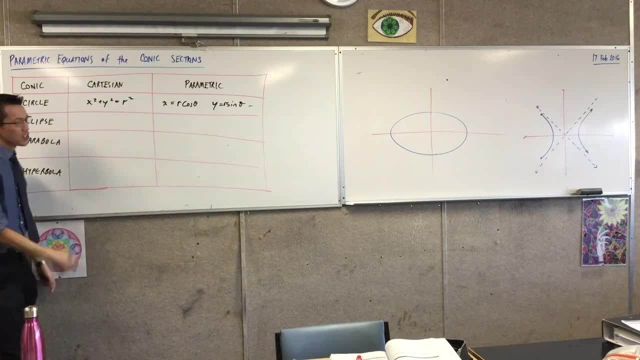 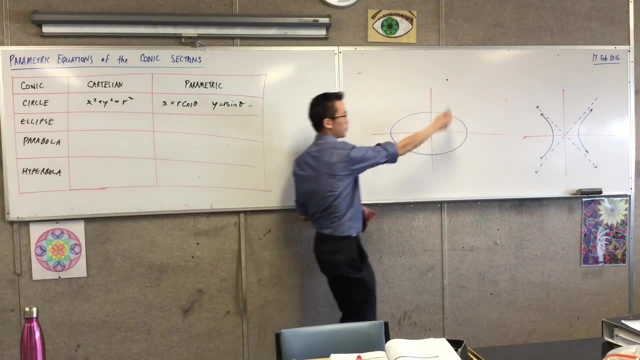 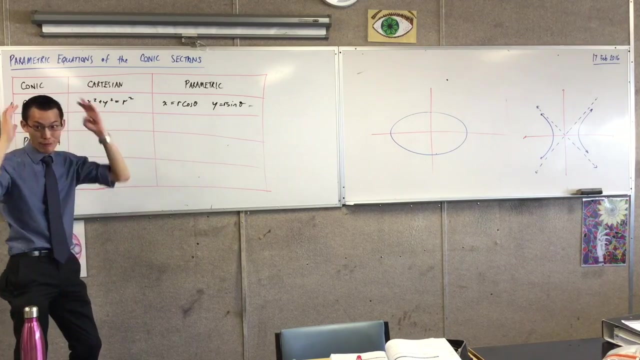 Like. so, Also important to mention, there's kind of a range restriction on theta right. It can't just go anywhere, Because once you go like around a full revolution, you've come back to where you started, right. So therefore, I guess the way I would say this is as an extension to students thinking in gradients rather than in degrees. I can go from 0 to 2 pi. That's one full revolution. I mean, in theory, there's nothing stopping you from going past 2 pi, But the whole point is to have one unique defining factor for where you are on your locus, right. 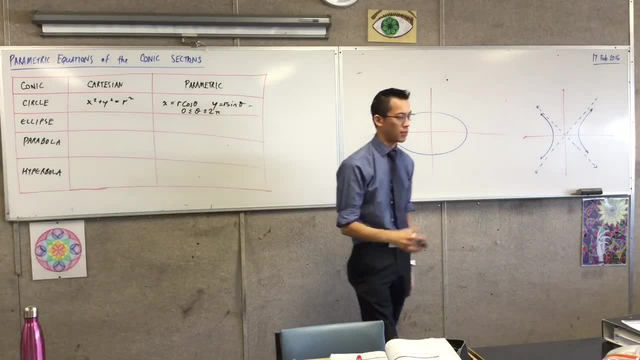 So, therefore, if I restrict it from 0 to 2 pi, everything is unique, Uniquity, Uniquity. Okay. So when we go to the ellipse, what changes? Okay, We still have the x-squared plus y-squared. 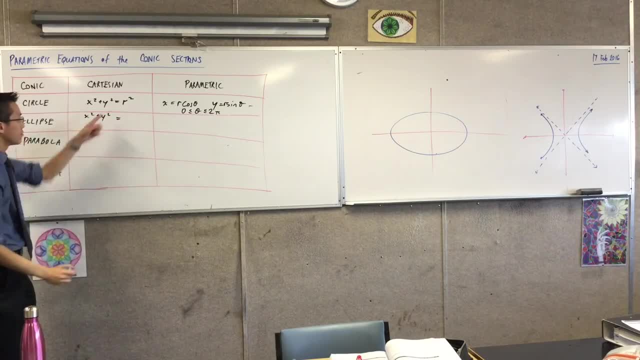 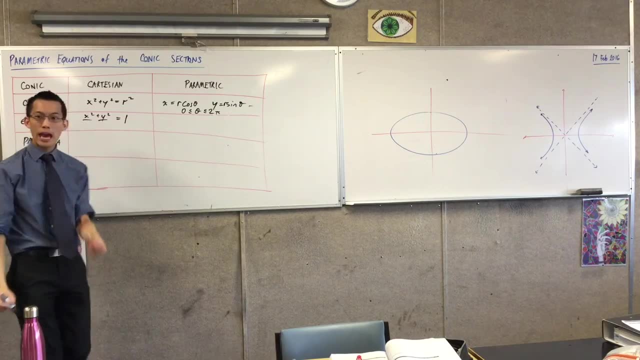 But we don't frame it in these terms, do we? We tend to say: well, there's a 1 over here, And then we get some denominators And we have different denominators, generally speaking, because if you don't have different denominators, you're back up in circle territory. 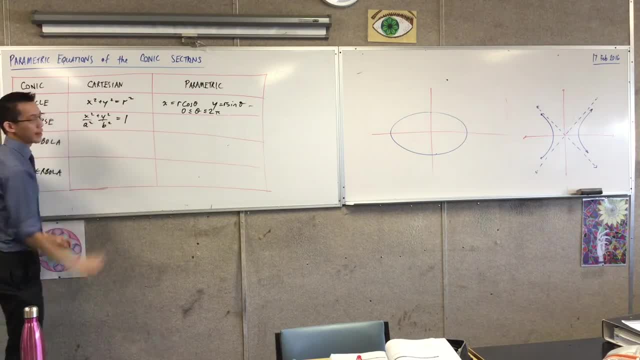 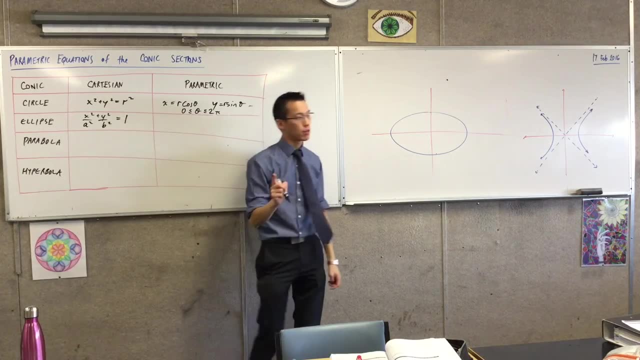 Yes, So we've got our a-squared and our b-squared here, And here's one of the beauties of parametric forms, right? Because what this does is this: takes the unit circle right: x squared plus y squared equals 1, and it stretches the 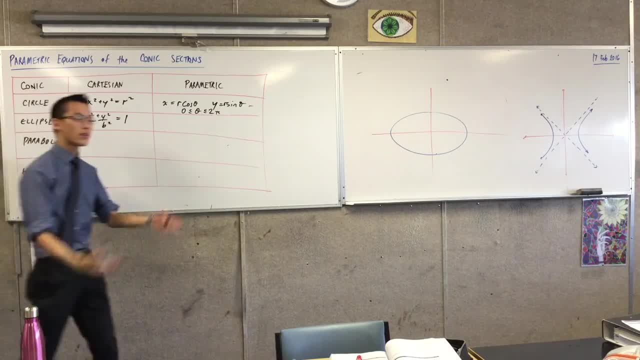 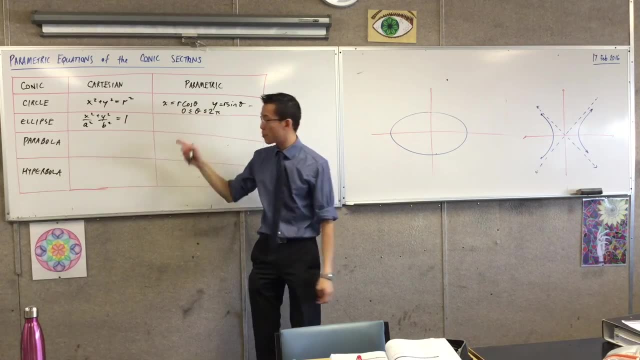 So we've got our a2 and our b2 here, And here's one of the beauties of parametric forms, right? Because what this does is this: takes the unit circle right- x squared plus y squared equals 1, and it stretches the. 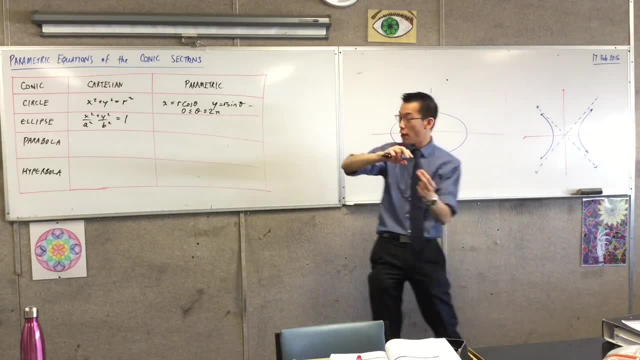 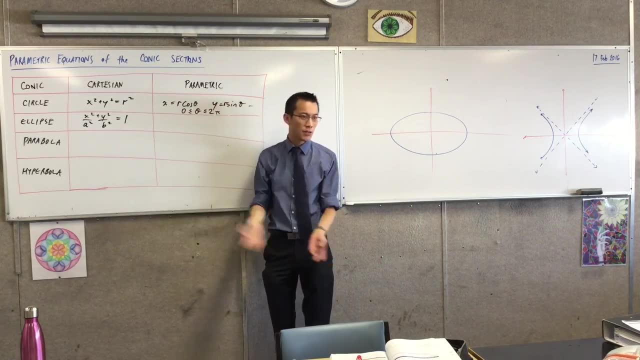 horizontal out a times bigger and it stretches the vertical out b times bigger right. So, instead of being a cos theta sine theta, There's no r to speak of because it doesn't have a radius right. You're going to be at x equals. 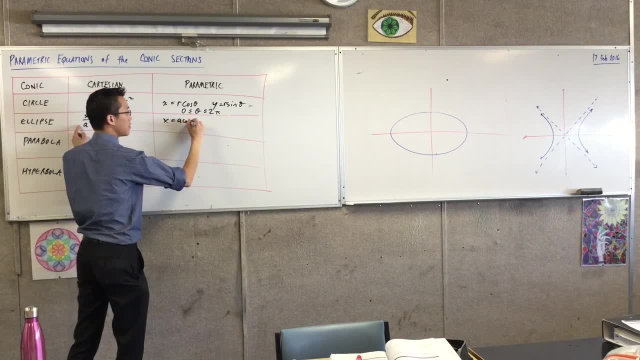 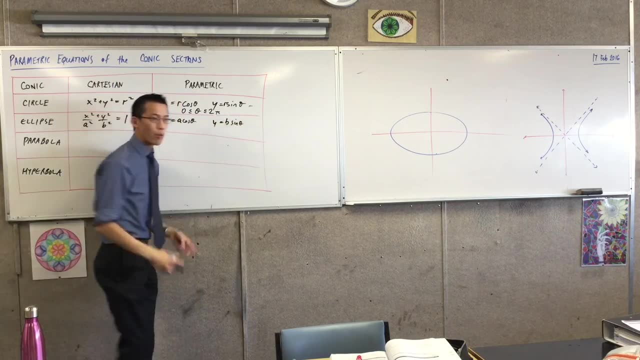 you'll be a times further away from the origin. so you get a cos theta and And you'll be b times further than the origin, speaking vertically. so you'll be at b sine theta right And we have the same restriction coming in: 0, theta 2 pi. 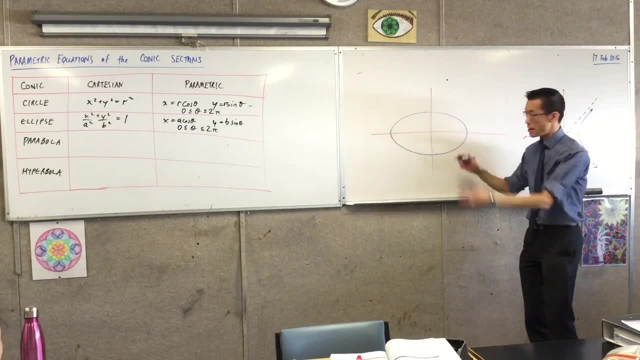 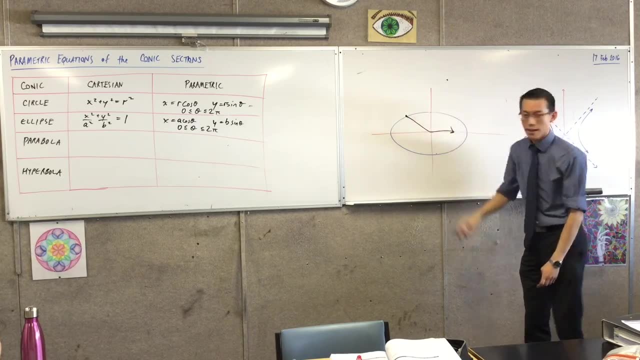 So you can see, I can just like I can on the circle, I can uniquely pick any point like say: there, right, And I can say, alright, Just measure the angle from that point to the positive. that's a pretty bad line. positive x-axis, You've got an angle there. 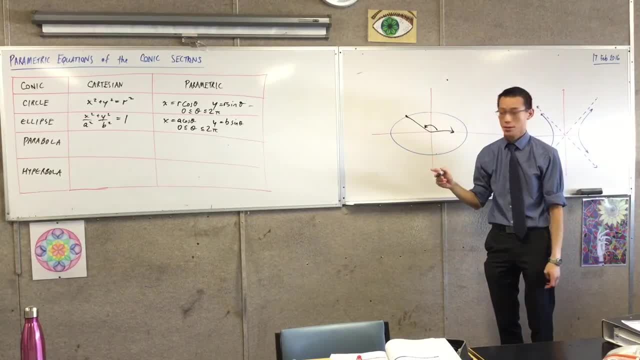 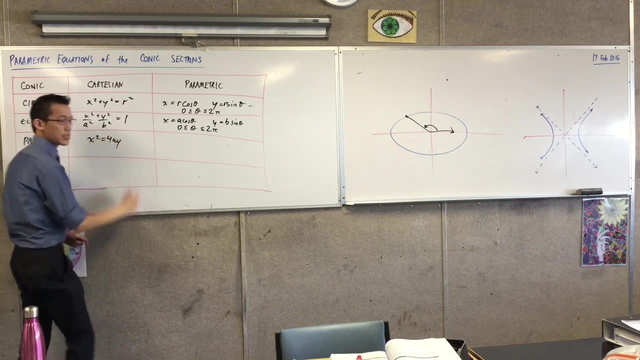 That's the single value. you need to know where you are on the ellipse. That's really good. Now the parabola. we dealt with the parabola a while ago. This Is the form that we would generally use to make the, the parameter, the parametric force, nice and neat, right. 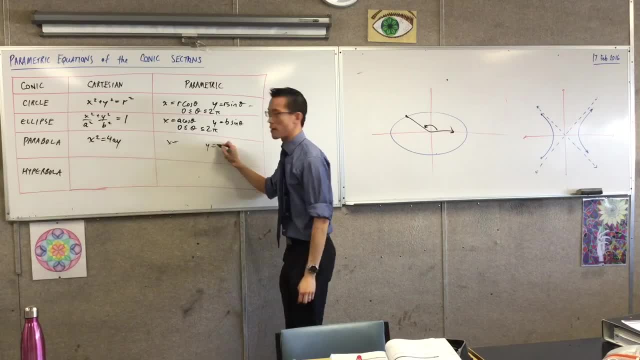 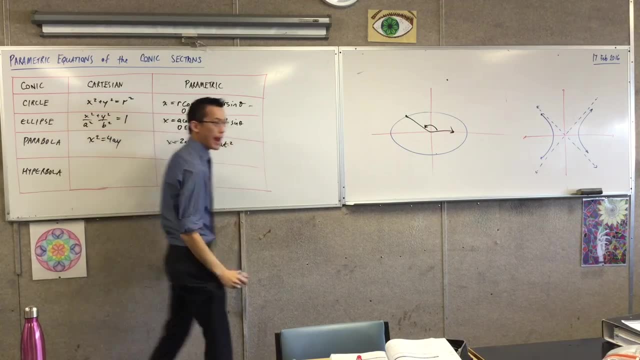 Who remembers what our x and our y are? What are you talking about? The parabola 2 a, t a, t squared. Very good, 2 a, t a t squared, and it's worth remembering that we've gone from angle territory. 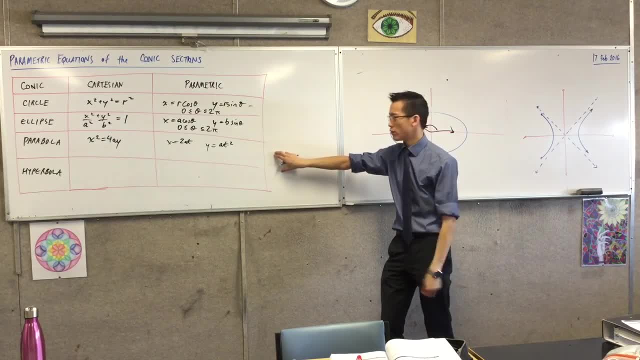 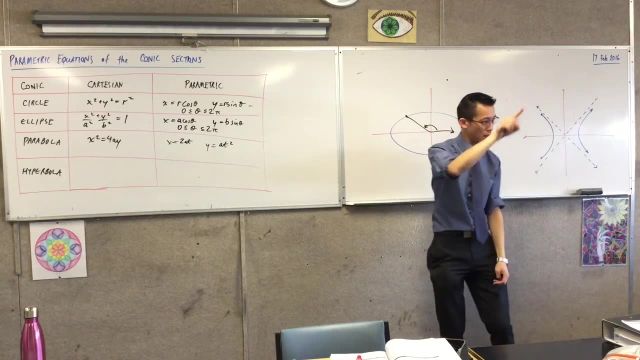 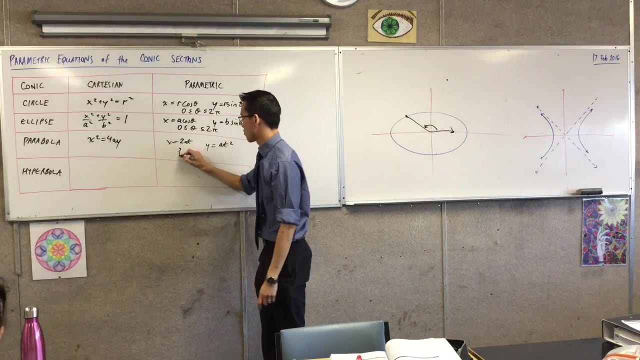 to here, where you honestly could define it by an angle, but it is more useful for us to define it as. what is the parameter? we chose The gradient right Because anywhere on the parabola right, Every point on the parabola always has a different gradient to every other point on the parabola. So therefore gradient. so I'll just 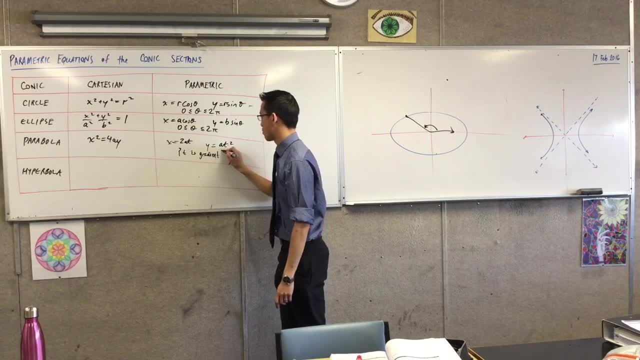 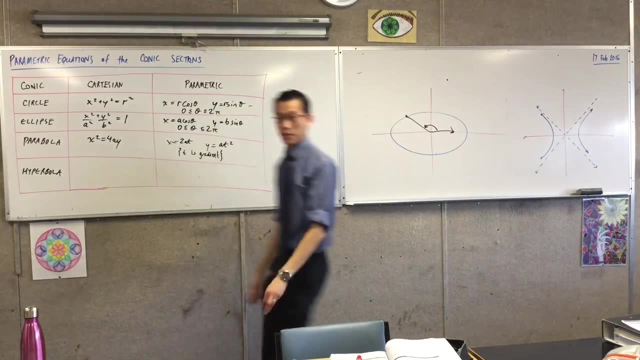 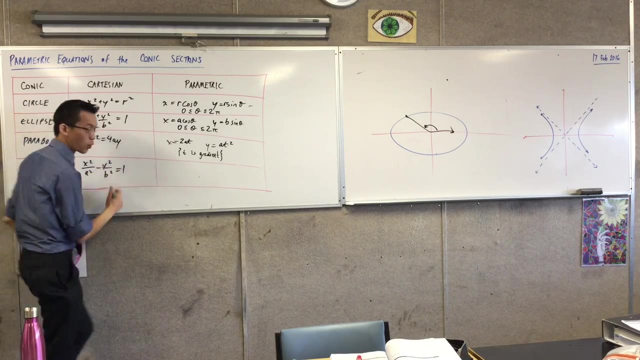 T is gradient. Gradient is a great thing to pick because it makes calculus easier, and all that. Now we come to the hyperbola. Okay, so we have a standard form: x squared on a squared, And of course we can switch around the x squared and y squared if you wanted a conjugate hyperbola. 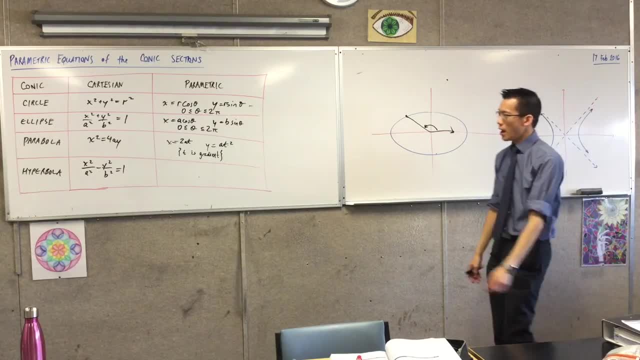 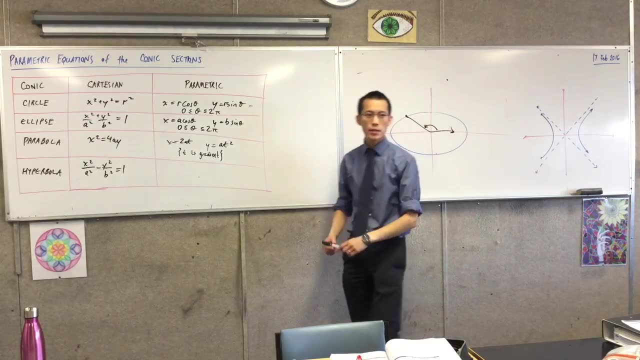 But I don't want to jump straight to what. what is the form? Okay, the first thing I want to point out is that here we had angles, then we went to gradient. Okay, you have a look at this. Is gradient going to be a good choice for defining where you are on the locus? 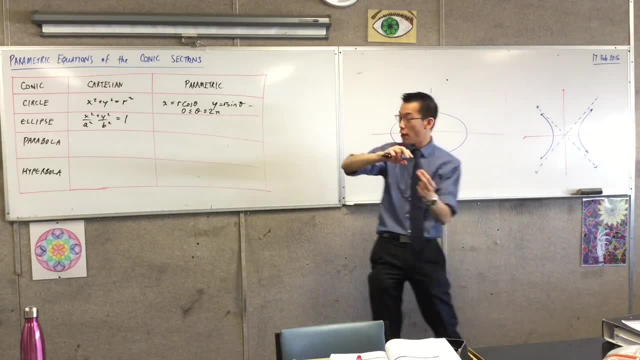 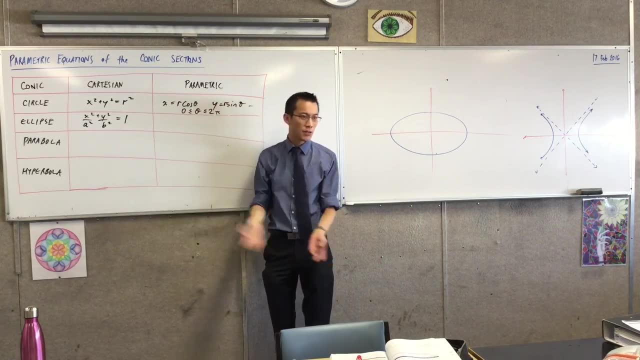 horizontal out a times bigger and it stretches the vertical out b times bigger right. So, instead of being a cos theta sine theta, There's no r to speak of because it doesn't have a radius right. You're going to be at x equals. 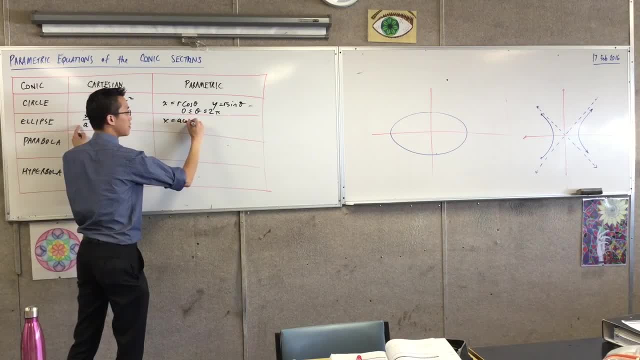 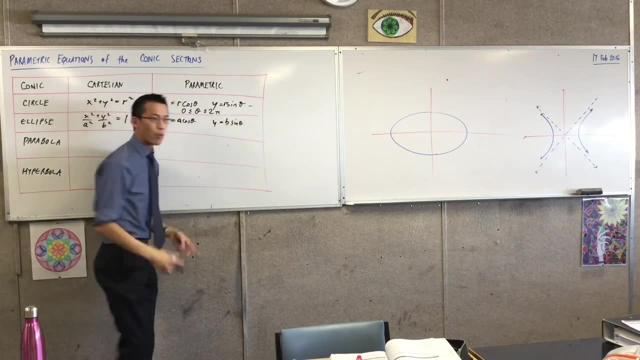 you'll be a times further away from the origin. so you get a cos theta and And you'll be b times further than the origin, speaking vertically. so you'll be at b sine theta right And we have the same restriction coming in: 0, theta. 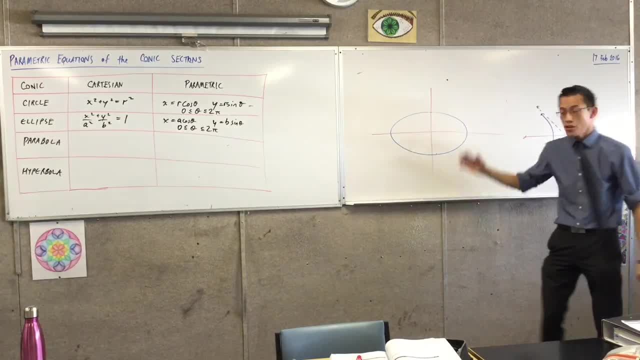 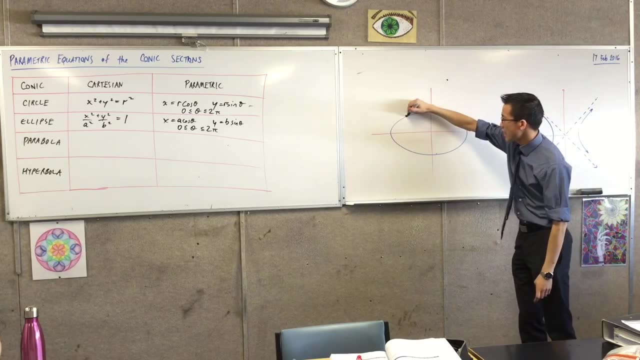 2 pi. okay, So you can see, I can just like I can on the circle. I can uniquely pick any point, like say there, right, And I can say, alright, Just measure the angle from that point to the positive. that's a pretty bad line. positive x-axis. You've got an angle there. 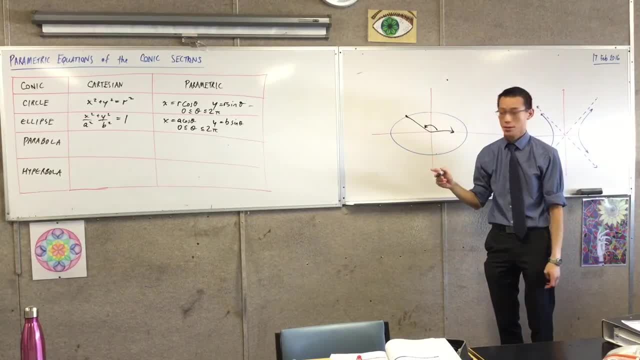 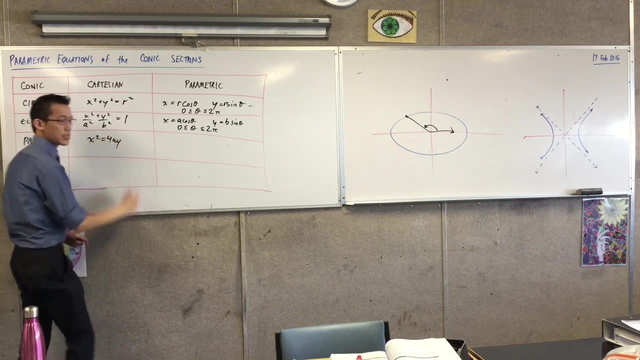 That's the single value. you need to know where you are on the ellipse. That's really good. Now the parabola. we dealt with the parabola a while ago. This Is the form that we would generally use to make the, the parameter, the parametric force, nice and neat, right. 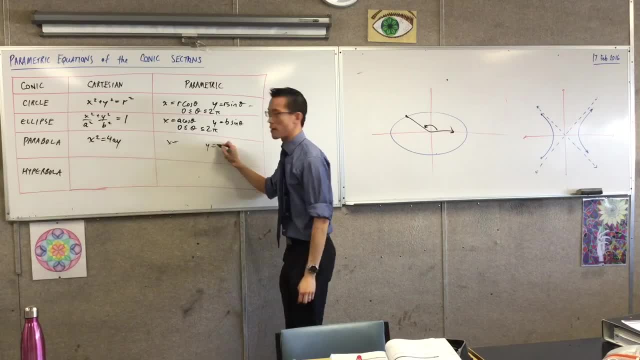 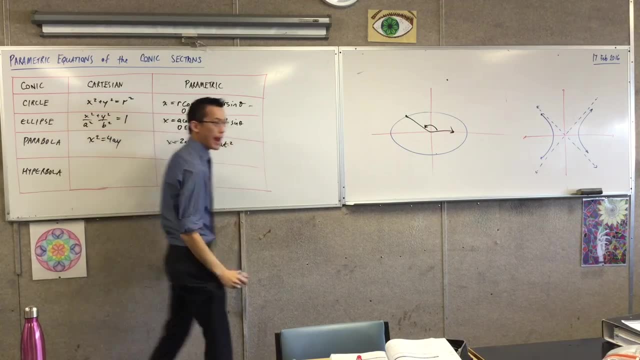 Who remembers what our x and our y are? What are you talking about? The parabola 2 a, t a, t squared. Very good, 2 a, t a t squared, and it's worth remembering that we've gone from angle territory. 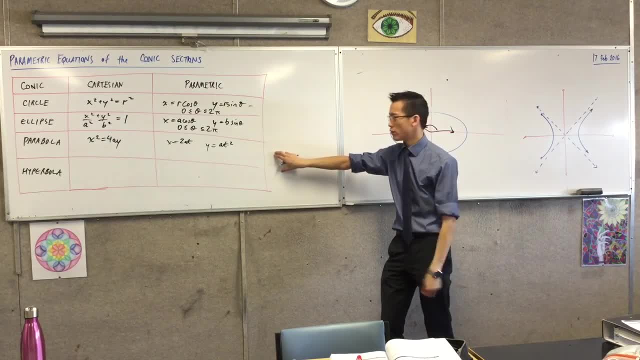 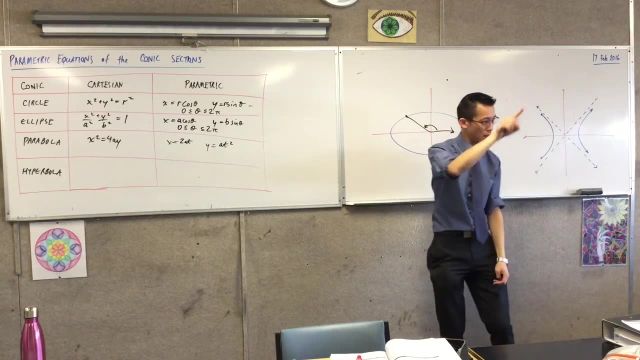 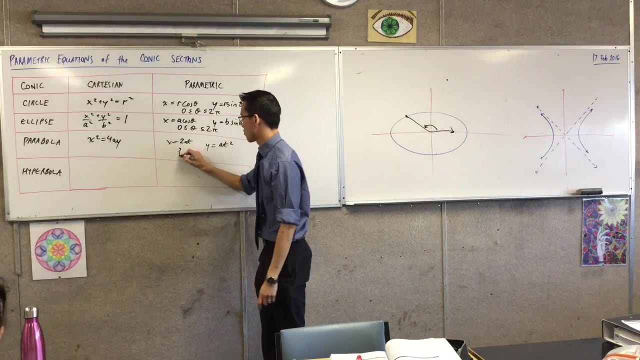 to here, where you honestly could define it by an angle, but it is more useful for us to define it as. what is the parameter? we chose The gradient right Because anywhere on the parabola right, Every point on the parabola always has a different gradient to every other point on the parabola. So therefore gradient. so I'll just 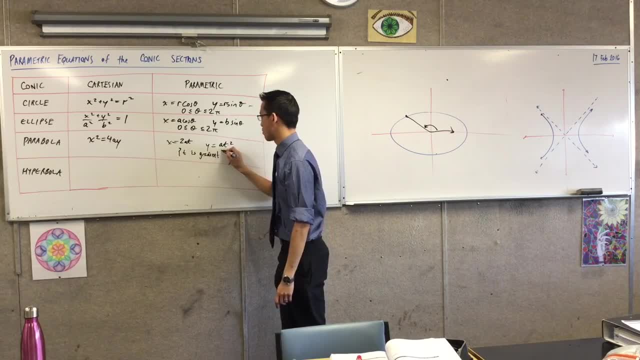 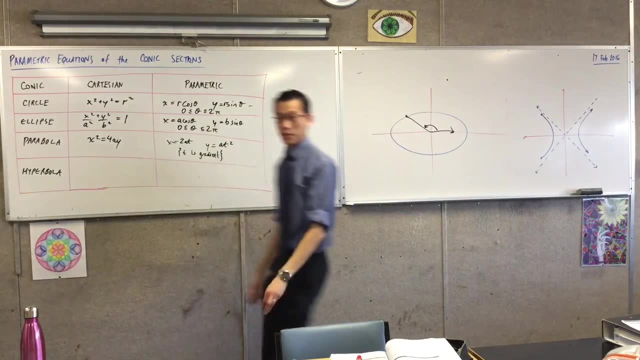 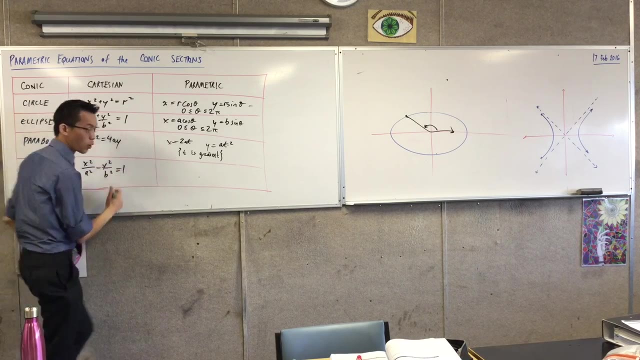 T is gradient. Gradient is a great thing to pick because it makes calculus easier, and all that. Now we come to the hyperbola. Okay, so we have a standard form: x squared on a squared, d squared Minus, and of course we can switch around the x-squared and y-squared if we wanted the conjugate hyperbola. 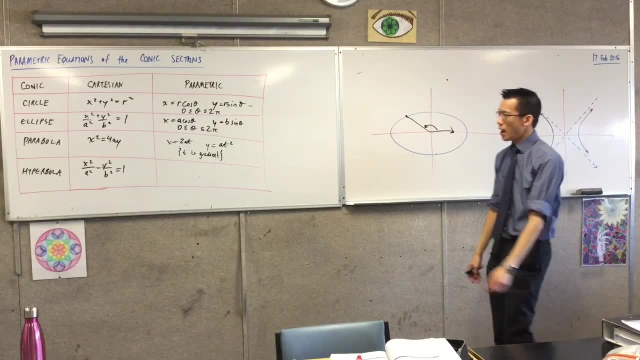 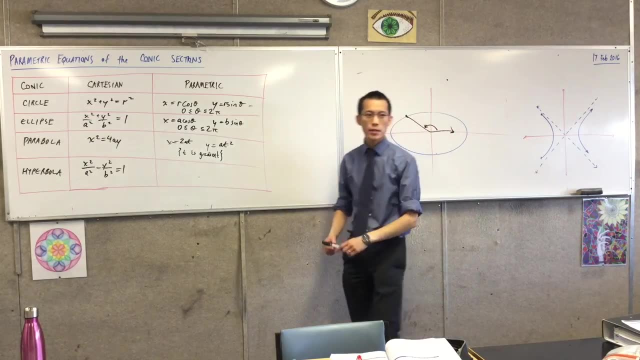 But I don't want to jump straight to what is the form. Okay, the first thing I want to point out is that here we had angles, then we've went to gradient. Okay, you have a look at this. is gradient going to be a good choice for defining where you are on the locus? 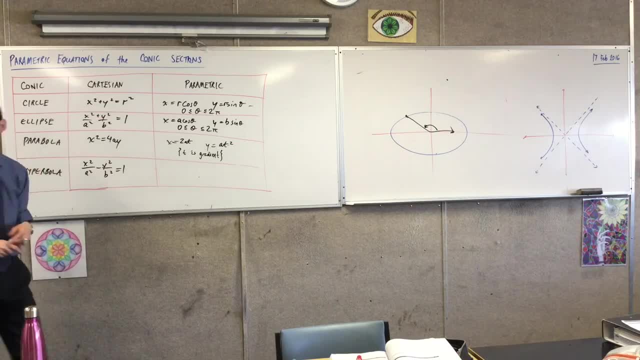 And the answer is no, not really because of all the crazy symmetry that you've got right. every point has a gradient, But it also has another point that shares exactly the same gradient right on the opposite side in the other quadrant. okay, so gradients going to be no good. how about angle? 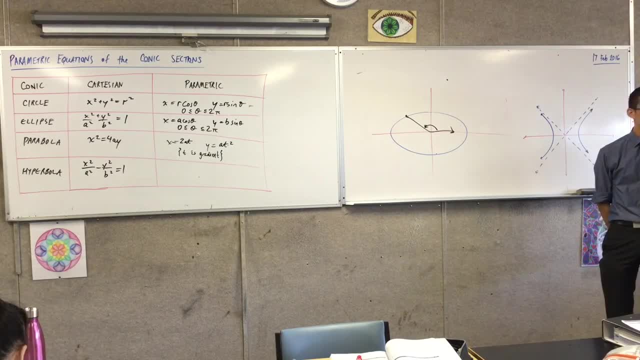 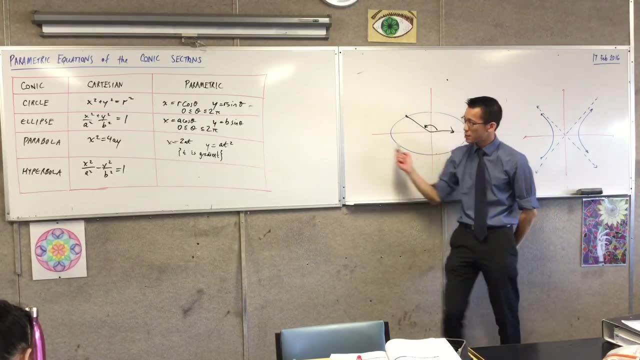 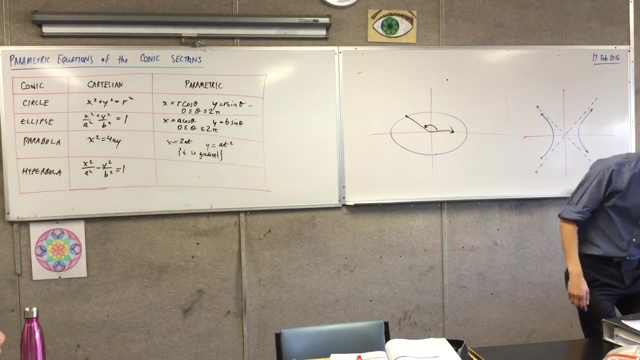 would angle work is every point uniquely defined by angle. now it is not nearly as obvious versus the ellipse and versus the circle, but if I- unfortunately I didn't have a ruler here- actually can I borrow someone's rule or diagram, spoiler this one's better and it will not involve my inability to catch, okay if I. 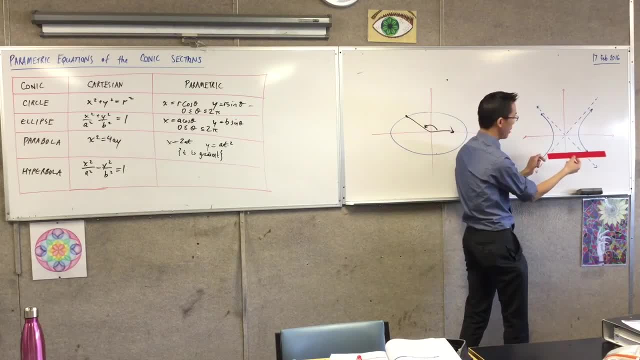 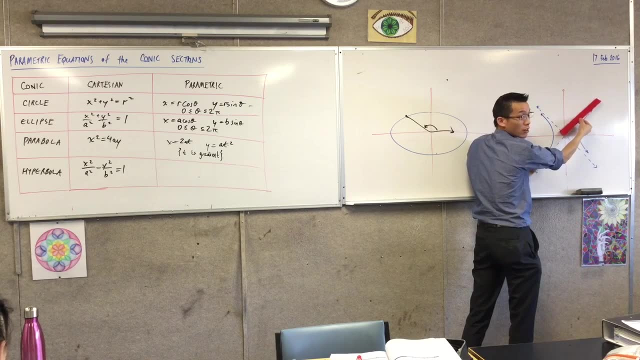 take this and I say, alright, vision from the origin, right, and remembering that like this isn't going, but maybe this is a better way to do it, right. so that would be like, say, zero, right, I can go up. I probably haven't hitting one point on the locus. do you agree with that? right, I can spin all the way over to here I'm. 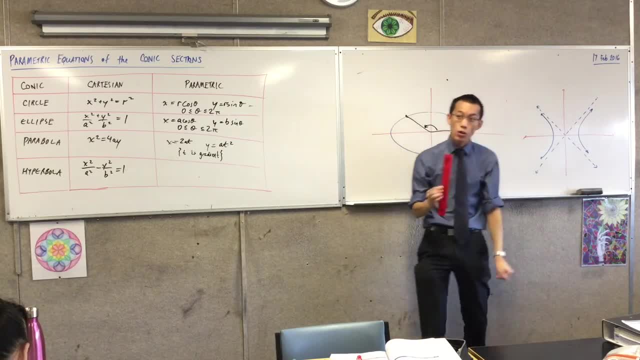 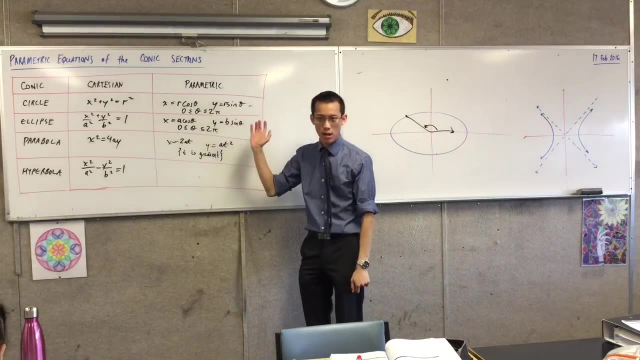 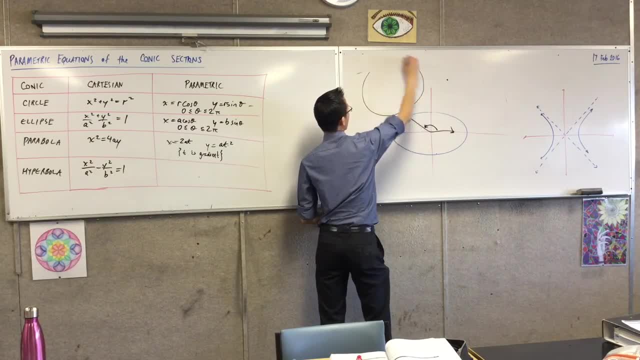 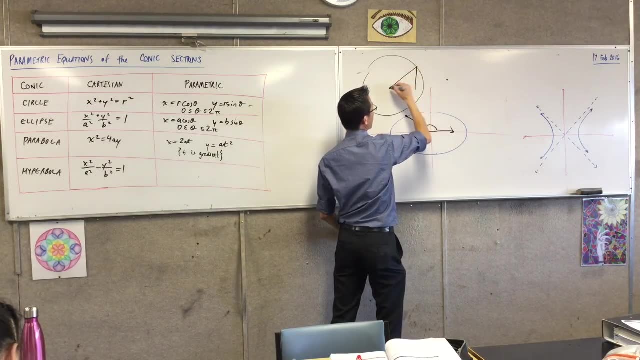 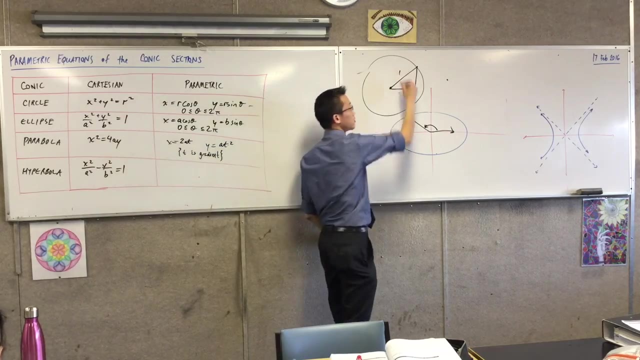 for the circle. in the circle from the center, what we measured was there's a point up there on the locus, and then we said, okay, well, there's a right angle triangle hiding there. do you remember that? obviously we didn't start with a circle of any radius, we started with the unit circle right. this is your x. 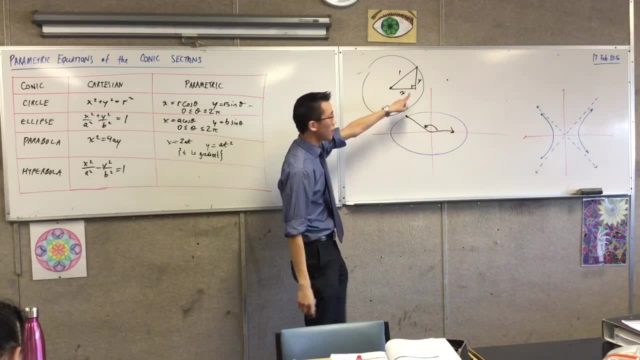 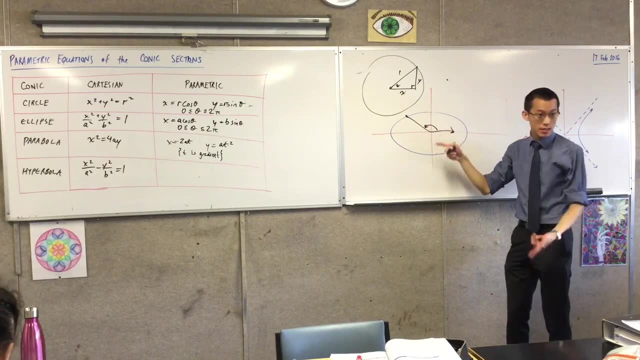 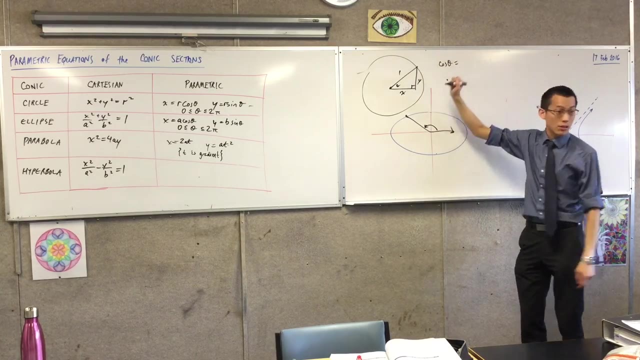 coordinate. this is your y coordinate. okay, now do you see out of here how these guys emerge? do you see it right? have a look, if I define that angle that we talked about here as a speed up, right in that right angle triangle, cos X, sorry, cos theta is equal. 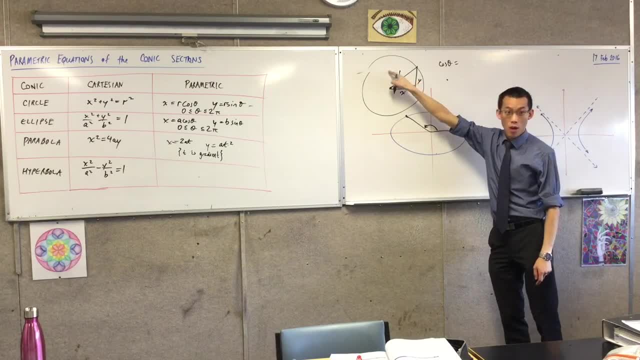 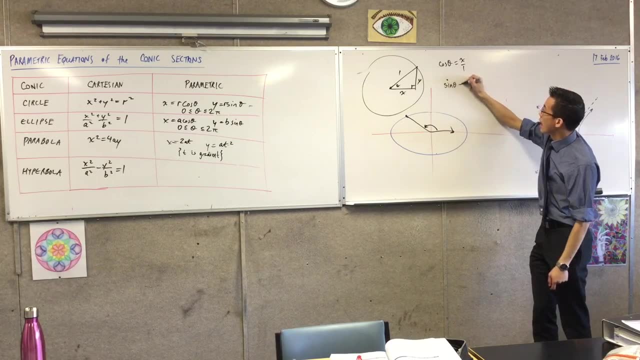 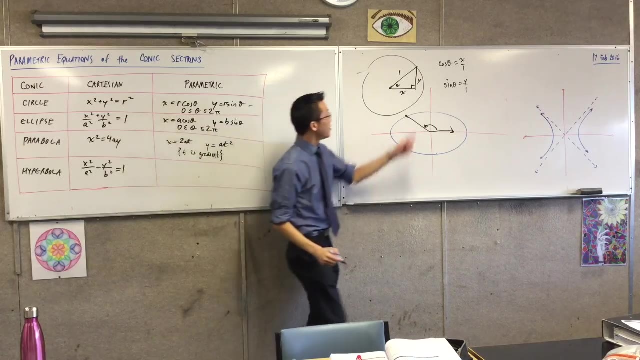 to x on 1 right adjacent on hypotenuse, so that's where your x equals cos theta comes from. and then, likewise, you get this relationship and of course you scale it up by R to get to this arbitrary circle. now that's really nice, because then you carry that forward from here, right? this of course makes sense. 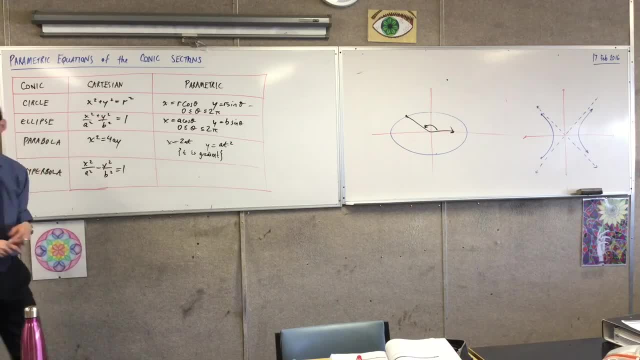 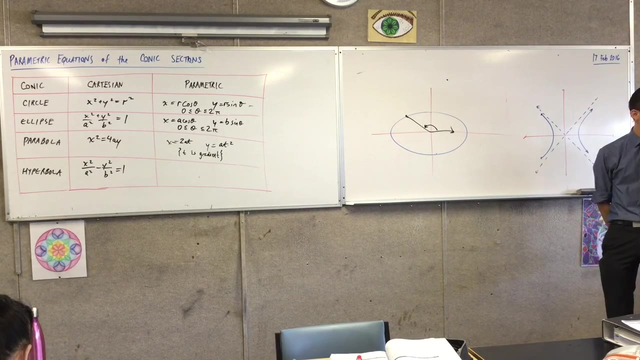 And the answer is no, not really Because of all the crazy symmetry that you've got right. Every point has a gradient, But it also has another point that shares exactly the same gradient right on the opposite side, in the other quadrant. Okay, so gradients going to be no good. How about angle? Would angle work? Is every point uniquely defined by angle? 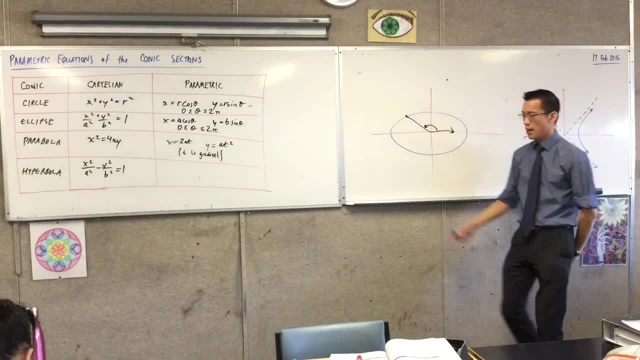 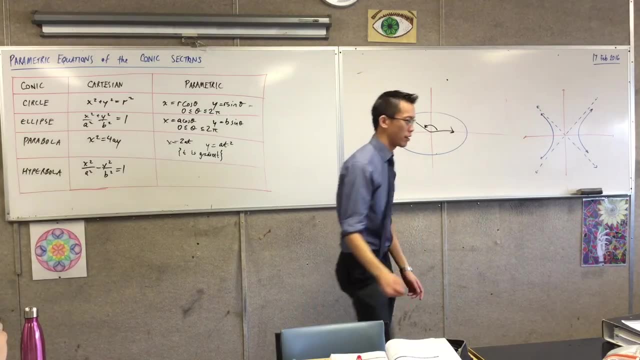 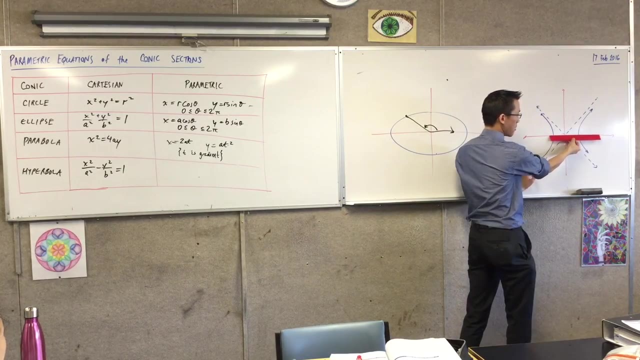 Now it is not nearly as obvious Versus the ellipse and versus the circle, but if I- unfortunately I didn't have a ruler here. Actually, can I borrow someone's ruler If I take this and I say, all right, this is for the origin, and remembering that like this isn't going. 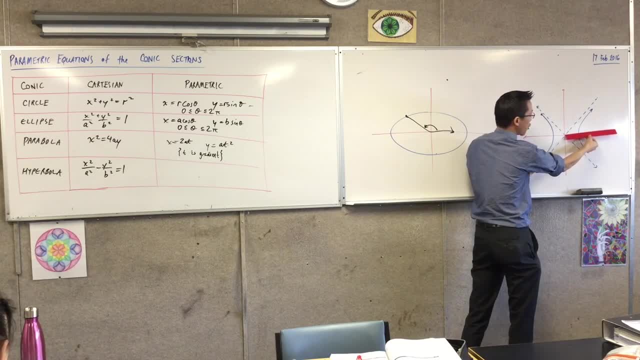 But maybe this is a better way to do it. So that would be like, say, zero, right, I could go up. I've only ever hitting one point on the locus. Do you agree with that? I can spin all the way over here, I'm still hitting only one point on the locus. It's working out. Angle will be fine. 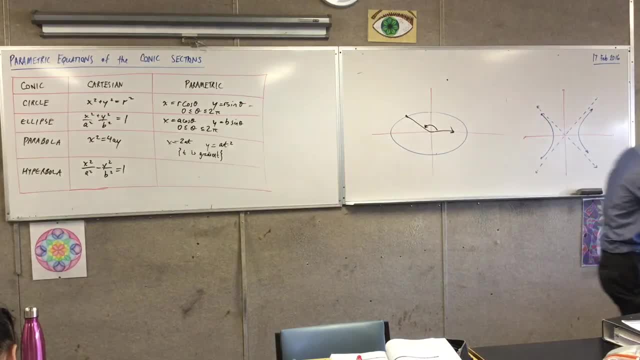 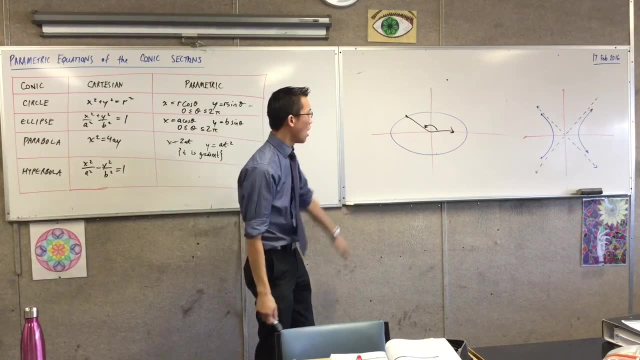 It'd be better than gradient, for sure. So how do I then use that? What equations? It's obviously not going to be cosin sine. So how do I arrive at this? Okay, now, rather, just hand them to you. I want you to remember how we did for the circle in the circle. 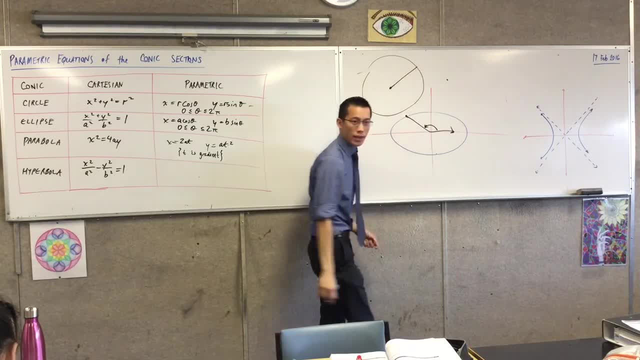 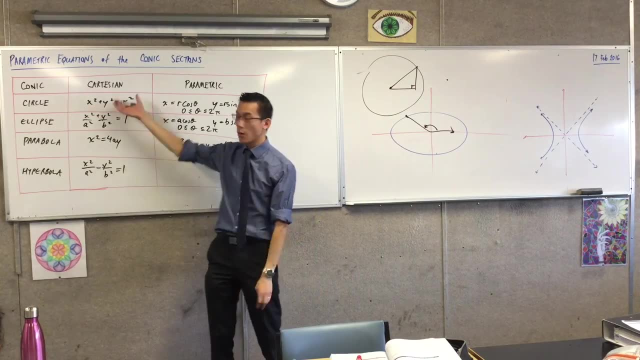 Well, in the center, What we measured was there's a point up there on the locus, and then we said, okay, Well, there's a right angle triangle hiding there. Do you remember that? Obviously, we didn't start with a circle of any radius, We started with the unit circle right. 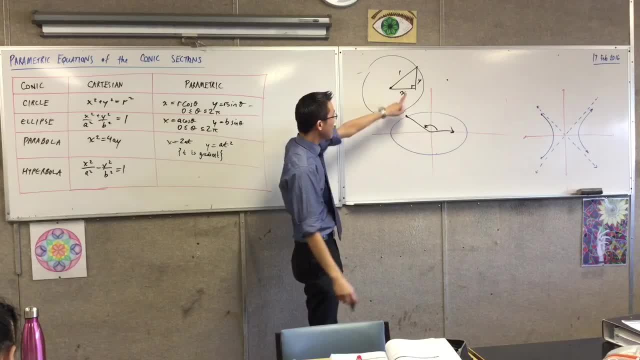 This is your x coordinate. This is your y coordinate. Okay, Now do you see out of here How these guys emerged? Okay, so this is your x coordinate. This is your y coordinate. Now do you see out of here how these guys emerged? 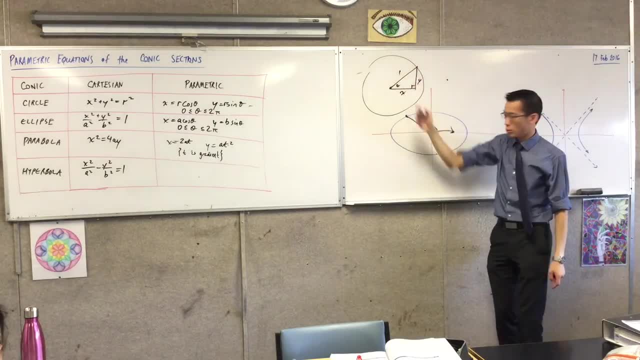 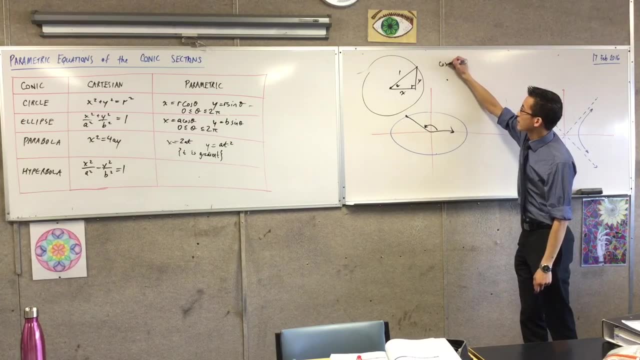 Do you see it Right? Have a look, If I define that angle that we talked about here as theta right in that right angle triangle, Cos x, sorry, cos theta is equal to x on 1, right Adjacent on. 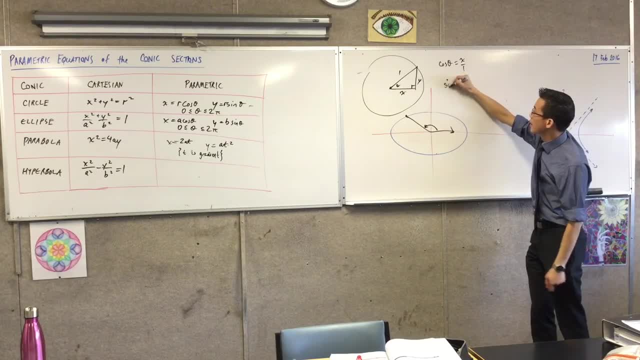 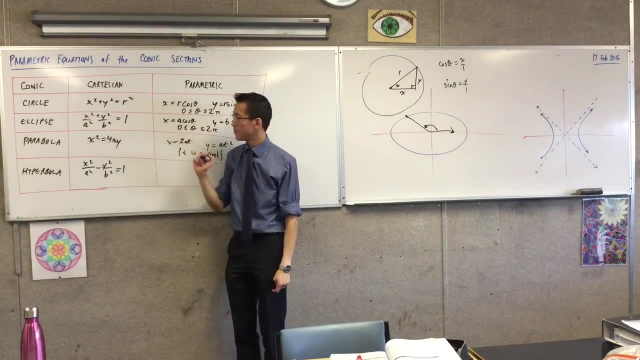 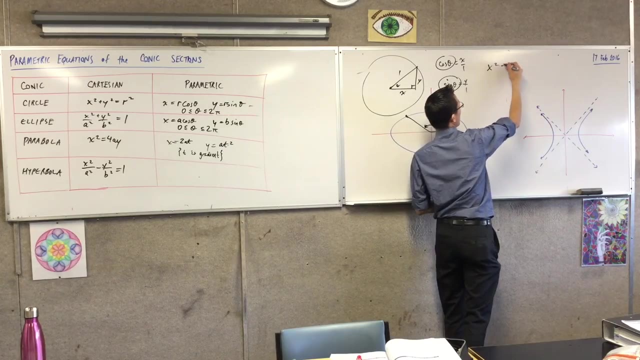 hypotenuse. so that's where your x equals cos theta comes from. and then, Likewise, you get this relationship and of course, you scale it up by r to get to this arbitrary circle. Okay, now that's Really nice, because then, if you carry that forward from here, right, This of course makes sense because you have this kind of shape. 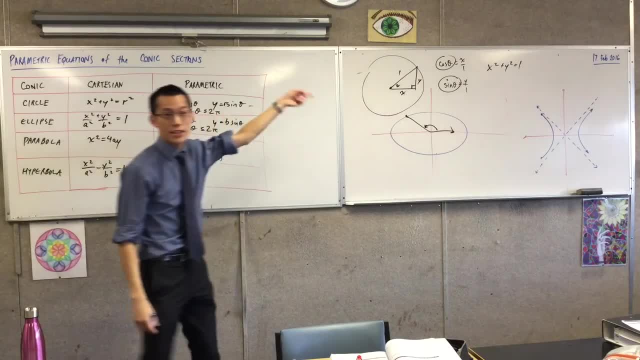 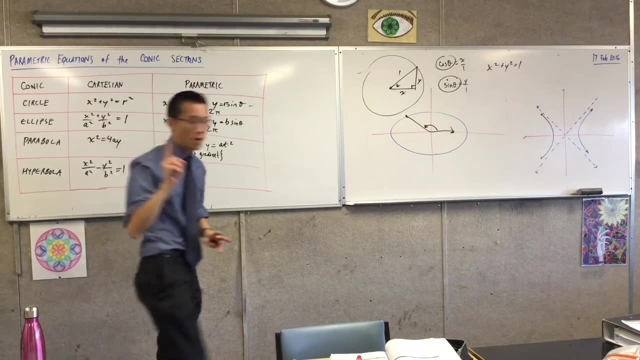 This is kind of equation I should say right, And the Pythagorean identity fits that perfectly. right. sine squared plus cos squared. I should say: cos squared plus sine squared equals what Happy. But we're now trying to deal with this.